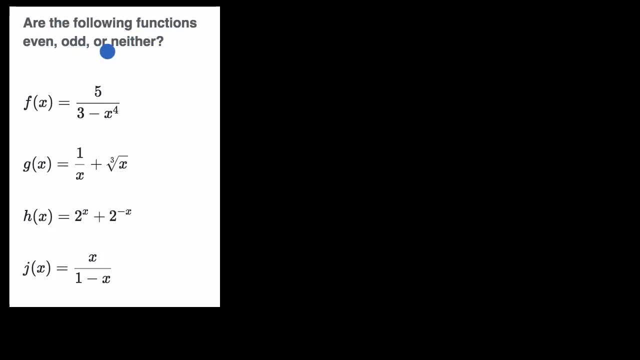 We are asked: are the following functions even, odd or neither? So pause this video and try to work that out on your own before we work through it together. All right, now let's just remind ourselves of a definition for even and odd functions. 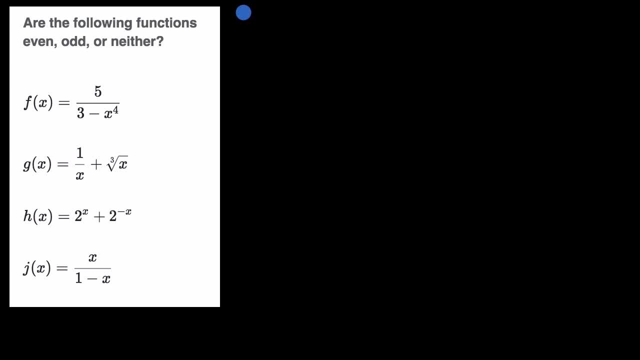 One way to think about it is what happens when you take f of negative x. If f of negative x is equal to the function again, then we're dealing with an even function. If we evaluate f of negative x instead of getting the function, 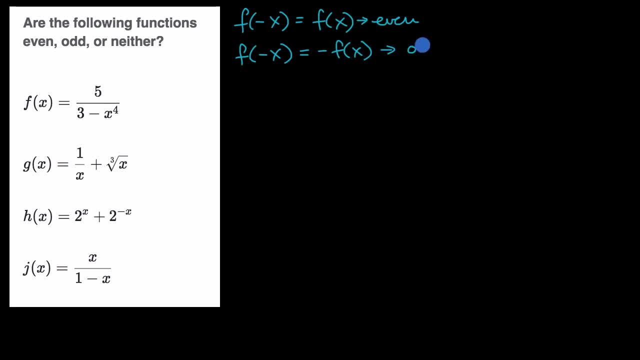 we get the negative of the function, then we're dealing with an odd function. And if neither of these are true, it is neither. So let's go to this first one right over here. f of x is equal to five over three minus x to the fourth. 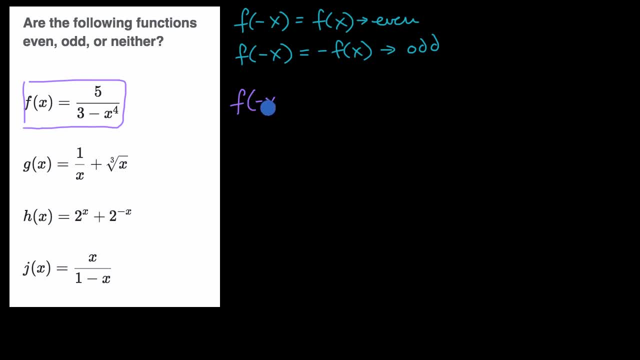 And the best way I can think about tackling this is: let's just evaluate what f of negative x would be equal to. That would be equal to five over three minus, and everywhere we see an x, we're going to replace that with a negative x. 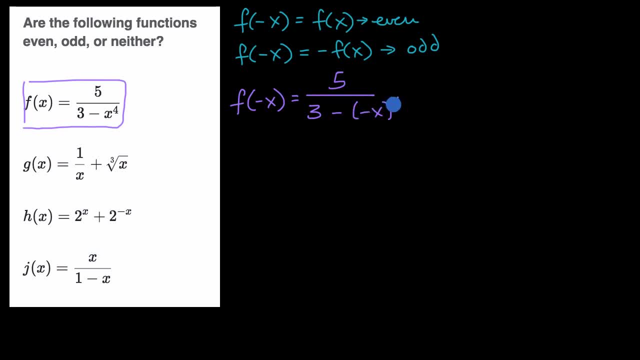 to the fourth power. Now, what is negative? x to the fourth power. Well, if you multiply a negative times a negative times a negative, how many times did I do that? If you take a negative to the fourth power, you're going to get a positive. 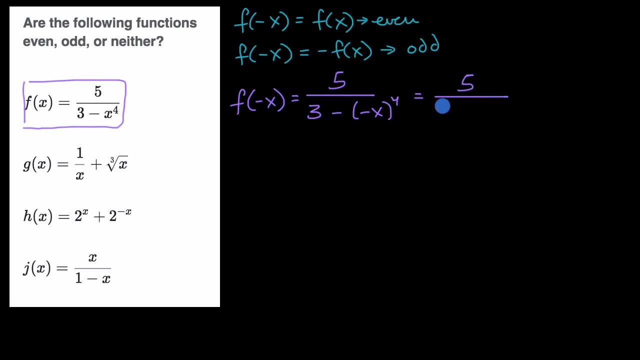 So that's going to be equal to five over three minus x to the fourth, which is once again equal to f of x. And so this first one right over here, f of negative x, is equal to f of x. it is clearly even. 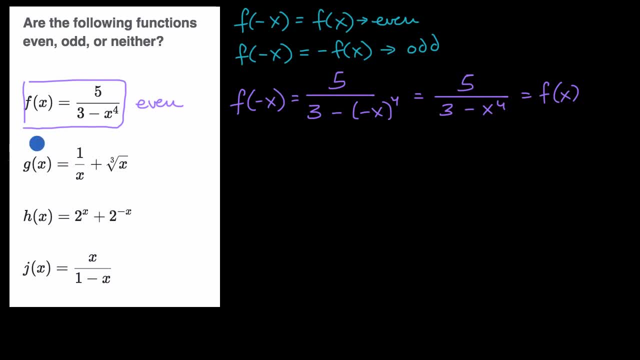 Let's do another example, So this one right over here: g of x. let's just evaluate g of negative x. And at any point you feel inspired and you didn't figure it out the first time, pause the video again and try to work it out on your own. 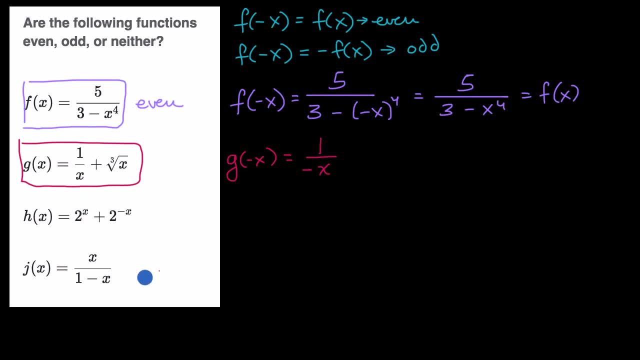 Well, g of negative x is equal to one over negative x, plus the cube root of negative x. And let's see, can we simplify this any? Well, we could rewrite this as the negative of one over x, And then I could view negative x as the same thing. 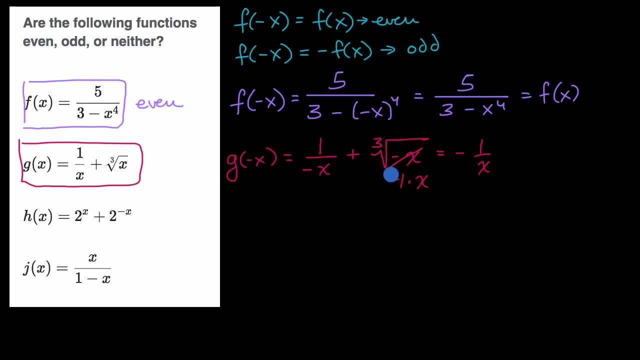 as negative one times x. And so we can factor out, or I should say we could take the negative one out of the radical. What is the cube root of negative one? Well, it's negative one, So we could say minus, we could say minus one.